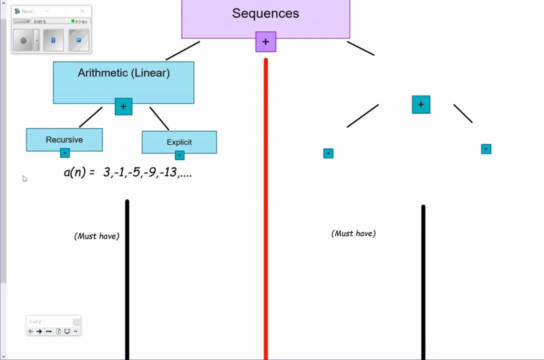 sequence something like this: a sub n equals 3 negative 1 negative 5, etc. and after investigating that a little bit, you should notice that it is decreasing at a constant rate. it has what's known as a common difference, alright, so in this case, from term to term, it's decreasing by 4. okay, so we'll start with. 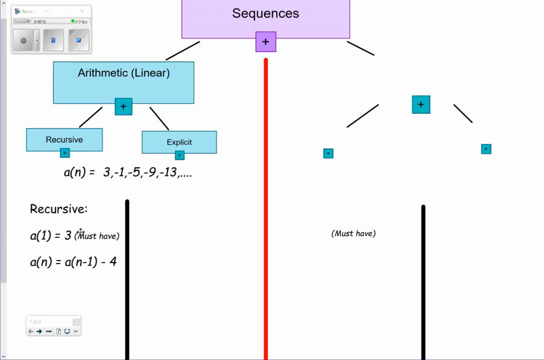 recursive. our recursive sequence is: Dassault-Roch, Bleu, okay, and in this case we our lemurs, we make 4 numbers. so this is our recursive sequence and very good, as you can see in our Mathemational, so that you get a term in between, which is dipping, which is your first term. 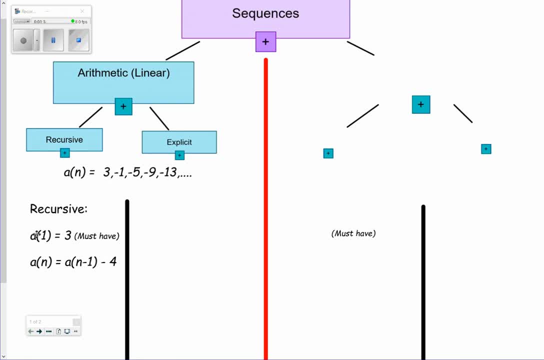 what you learn in our success TA in one in which you can't take any steps forward until you have the term before it. especially, you have to have that first term on your homework's. I notice a lot of you work including the first term in your recursive answers. you have to have that first term, okay. so what a sweatyjackander콕. 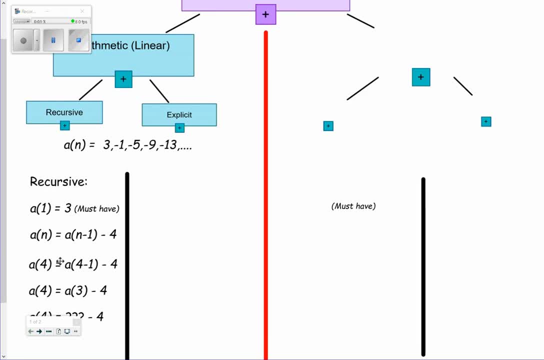 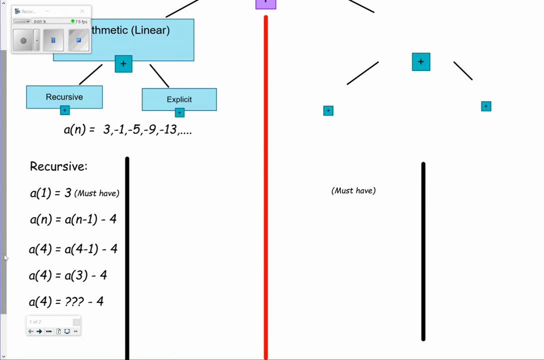 the point that you have to have the term prior Suppose with recursive. I just started out with saying, you know what I want: the fourth term. I have no idea what the second term is, or the third term. I just want to start right away and figure out what the fourth term is. Well, the reason it. 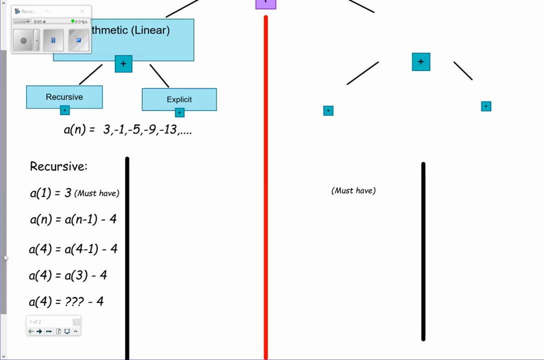 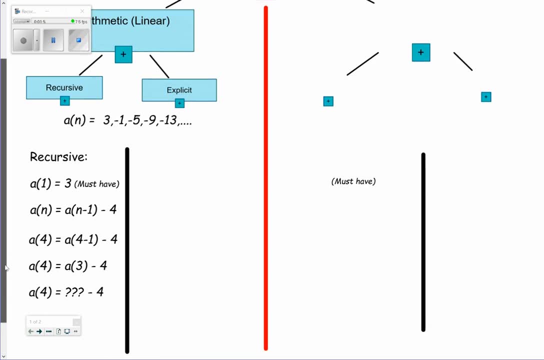 doesn't work for recursive sequences is this: Suppose I plug in a 4 for n, All right, I plug in a 4 for n here and a 4 for n here. Okay, at first it seems fine. a of 4 equals a of 3 minus. 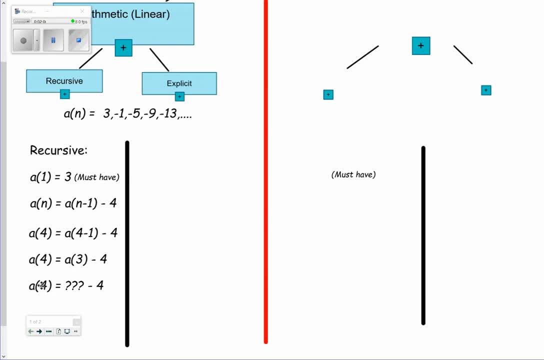 4. But at this step a of 4 equals. well, I don't know what the value of a of 3 is yet. I mean, yes, you can look up here, but suppose this was not here and you had to generate it. Okay, you can't. 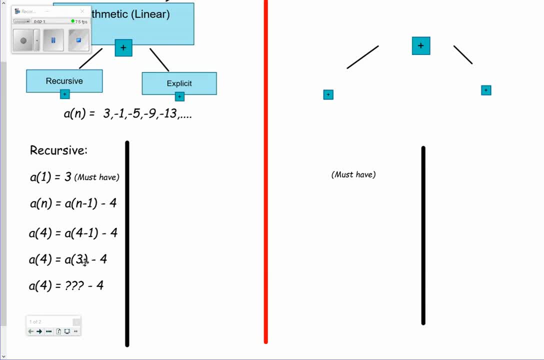 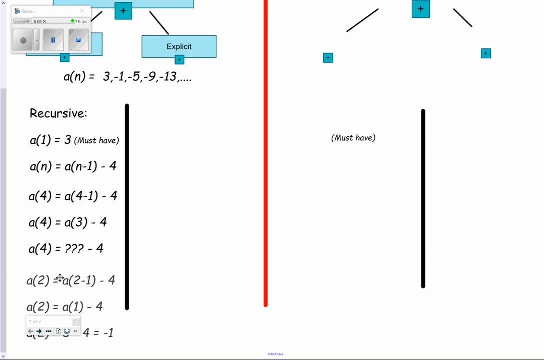 generate the third term, the fourth term until you have the third term. And I don't have the third term yet. Okay, so that's why, to properly apply a recursive sequence, it would go something like this: Okay, so I want the second. 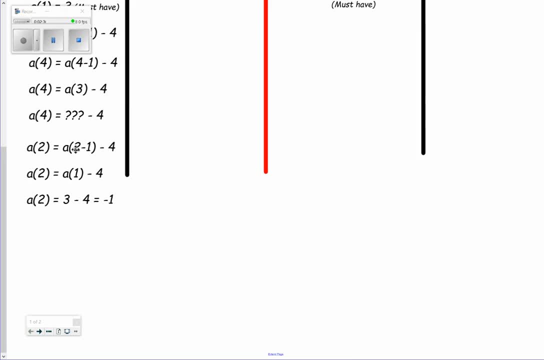 term. Okay, I'm going to plug a: 2 in for n here, 2 in for n here. 2 minus 1 is 1.. So the way I get the second term is I take the first term and subtract 4.. And that's cool, because I do have the. 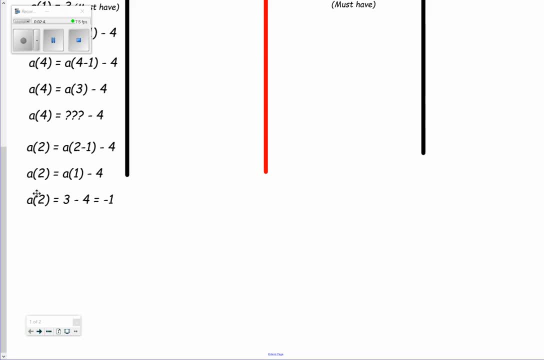 first term, in this case a 3.. So the second term is just the first term, subtract 4,, which is negative 1. And that matches the sequence. Okay, so that's a recursive Explicit says you can get to whatever term you want in a big, big hurry. 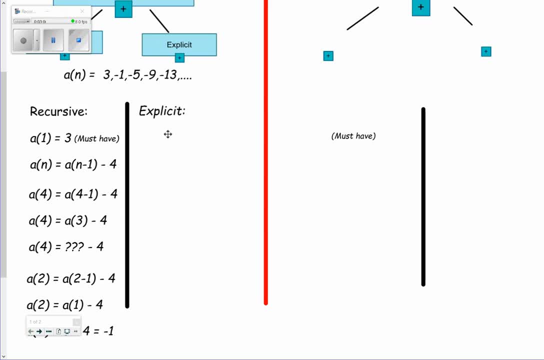 All right, this is the formula that's on your reference sheet. You do not need to memorize this. So suppose you had the general form of an explicit arithmetic equation off your reference sheet, which looks like this: Okay, the way you get a term is take the first term and add the term minus 1 times the common. 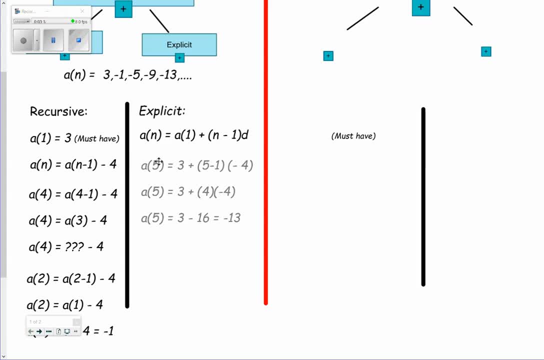 difference. Okay, so in this case suppose I wanted the fifth term. I'd plug a 5 in for n and I would plug a 5 in for n right here. All right again, the first term is 3.. And now just evaluate it: a of 5 equals 3 plus 4 times negative 4.. 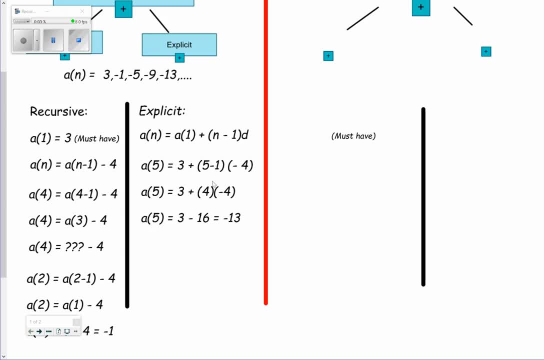 Right, again, this is 5 minus 1 times negative 4.. 4 times negative, 4 is a negative 16.. 3 subtract negative 16 is 13.. And it's the fifth term: negative 13.. 1,, 2,, 3, and it is Okay. so there's a brief. 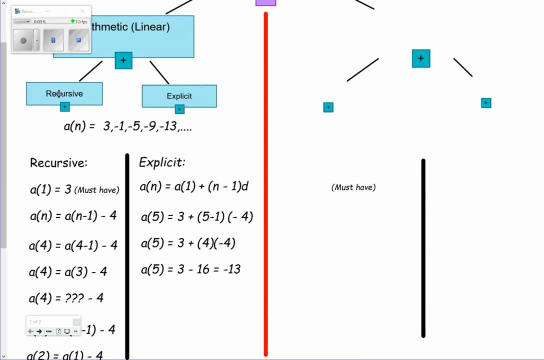 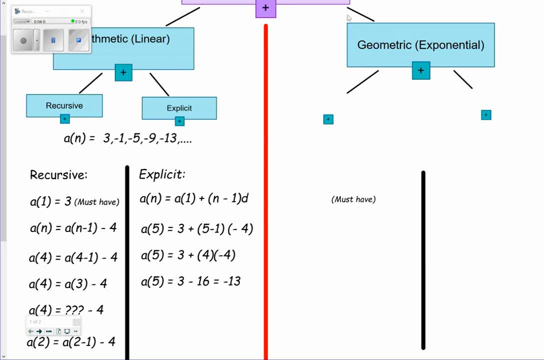 you an exponential curve, something we'll talk about more in the future, But for our purposes for right now, just think of it as a non-linear curve. So within geometric there is also recursive and explicit. So first recursive. So suppose you had to sequence something like this: 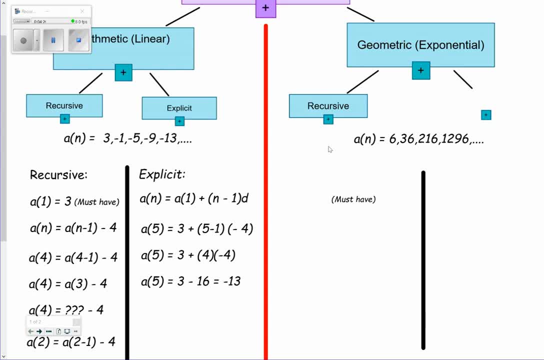 a of n equals 6, 36,, 216, 1296.. All right, so recursive with respect to geometric: Okay, Once again, you have to have that first term. If you don't have the first term, you are dead in the water. 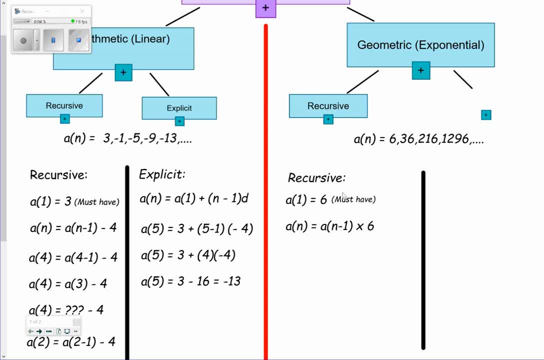 You can't go any further. So again, you have to have that. So what recursive geometric says is to get some term. okay, take the term before and multiply it by 6. All right, well, suppose I want the second term. 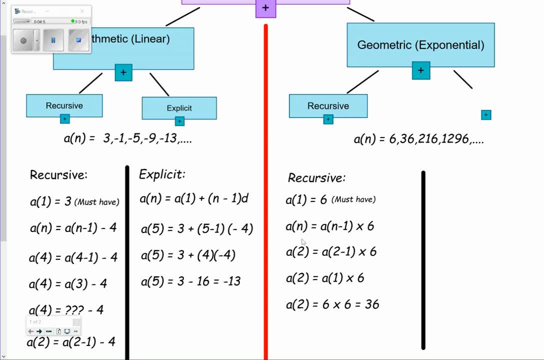 I take this: plug a 2 in for n here, plug a 2 in for n here. So the way I get a second term is: take the first term and multiply it by 6.. Well, what is 6 times 6?? 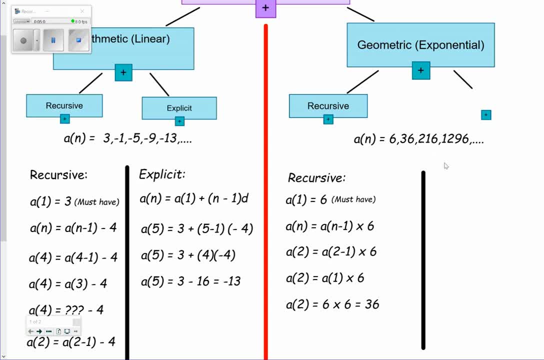 It's 36, and that does in fact give me the second term. Explicit once again says I can go wherever I want, Suppose I want to go with the whoops. sorry about that. So there's the general formula. 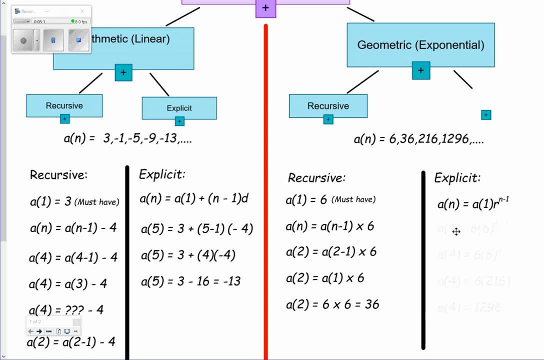 Again, that's on your reference sheet. You do not need to memorize it. So suppose I want the fourth term. Okay, I'm going to plug a 4 in for n here and a 4 in for n up in the exponent spot right here. 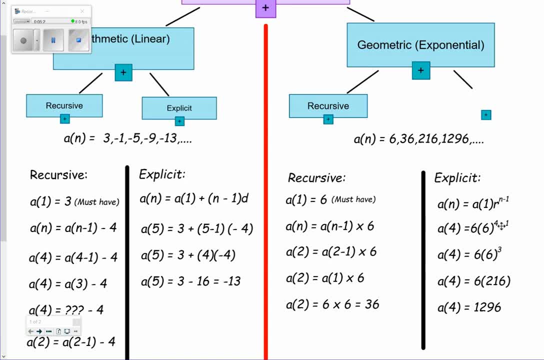 So I just take it one step at a time. The way I get the fourth term: 4 minus 1 is 3.. Okay, PEMDAS, 6 to the cubed or 6 to the third, power is 216,. 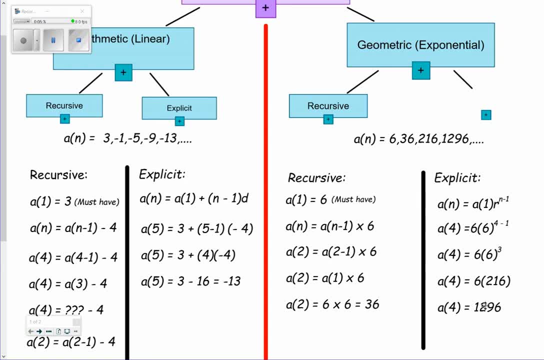 and 6 times 216 is in fact 1296, which is what we would expect, because that is the fourth term. Okay guys, whoop, here we go. Here's explicit Okay. so again within the mainframe of sequences: 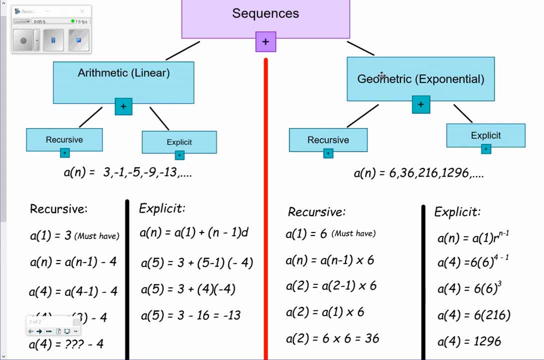 there's two major types: arithmetic and geometric, And then within each of those is recursive and explicit Explicit, which we just walked through. All right guys, hope that helped. Have a great day. Talk to you later. Bye. 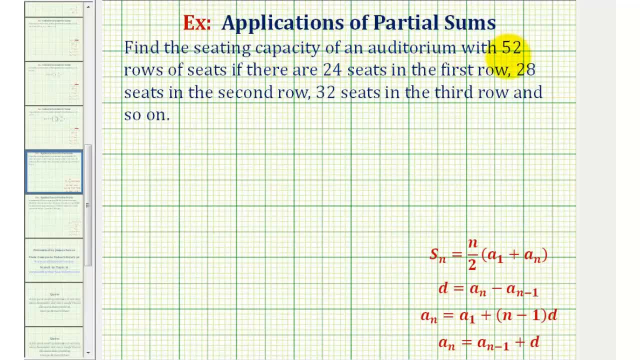 We want to find the seating capacity of an auditorium with fifty-two rows of seats if there are twenty-four seats in the first row, twenty-eight seats in the second row, thirty-two seats in the third row, and so on. We can model this situation using an arithmetic series. 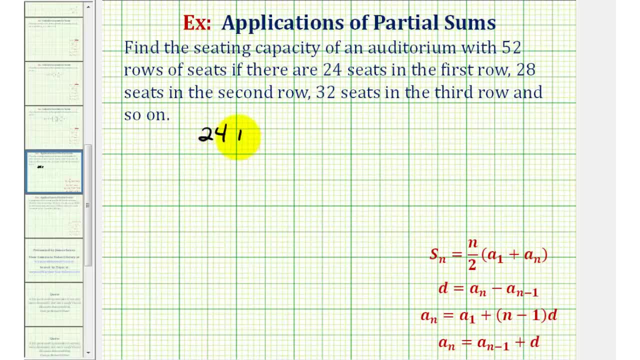 where the first term would be twenty-four plus the second term would be twenty-eight plus the third term, which would be thirty-two plus, all the way out to the fifty-second term, because there are fifty-two rows. There are several things we should notice here.